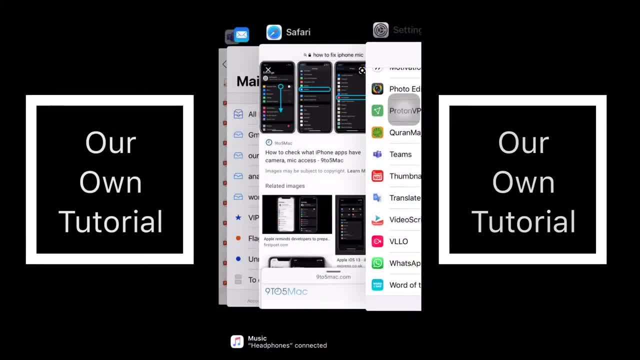 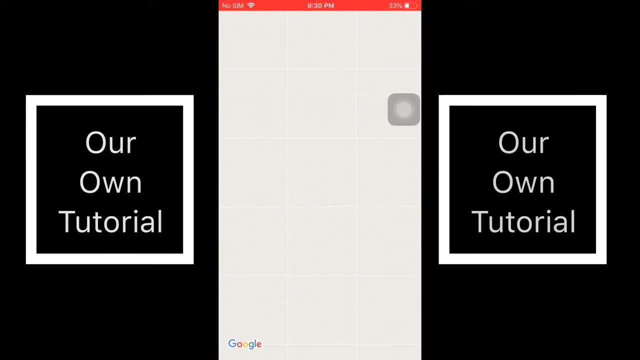 from the App Store. let me see whether have I removed the old one. okay, so open your Google map and wait for some time, let it be load in all the data and before measuring the distance, if you really want to change the unit of the distance, then also you can by using the Google map. 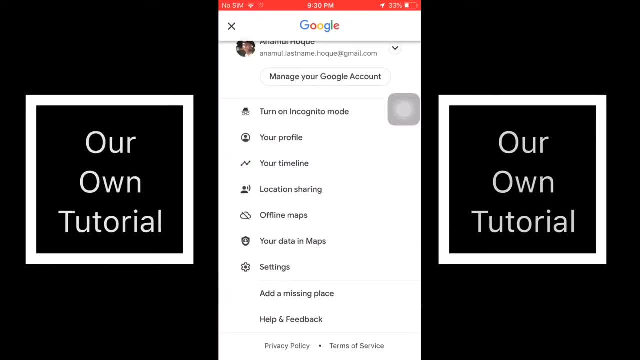 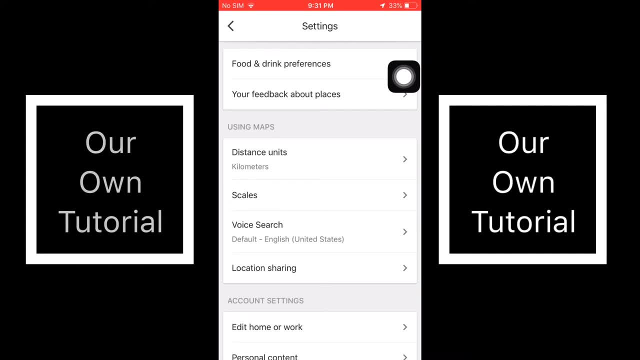 so just click on the profile and scroll down and then, as you can see, settings, just click on the settings and then scroll down the using the maps and then just click on the distance unit and you can choose like miles, kilometer, anything, whatever you like. so right now we're gonna measure the distance. well, I'm gonna. 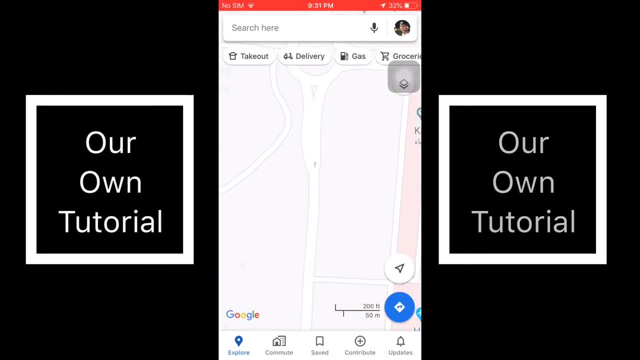 measure. I'm not gonna take that much long distance. I'm gonna measure till here, for example, till wait a minute. so till this way I will go, until come back in this way, okay, so first of all, the place, I mean place where you want to start measuring the 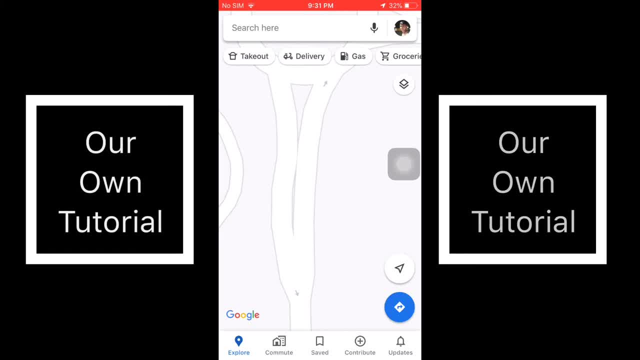 distance. just put your finger and just press it for some time until this red color button appear. so if you're using Android device, such as Samsung, then once this- I mean once this red color button appear over here, and then you will notice there is a drop to pin, so you do not have 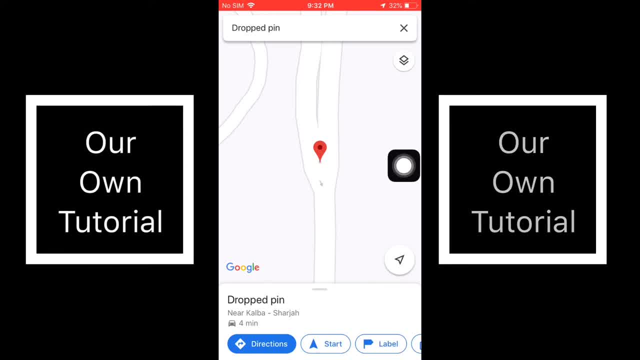 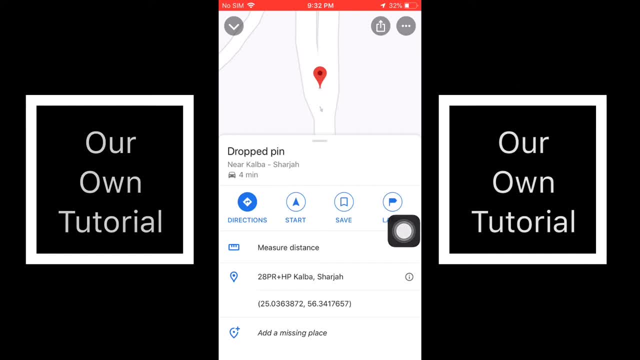 to scroll up, just click on it. in empty space, don't click on start level. this thing empty space. so once you click here, our for that Android also- just click on any kind of blur drop buttons will appear over there. just click on it. so from here you should have to click on measure the distance. so once you click. 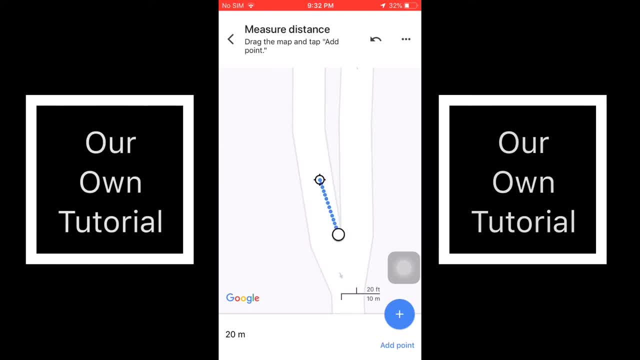 measure this distance now to make, this guy will appear over in your screens. so what you should have to do, for example, I just want to, I just want to measure till here by this way and then just click on plus button and then just move here. okay, all right, okay, then I will move this way. it's too much small and as 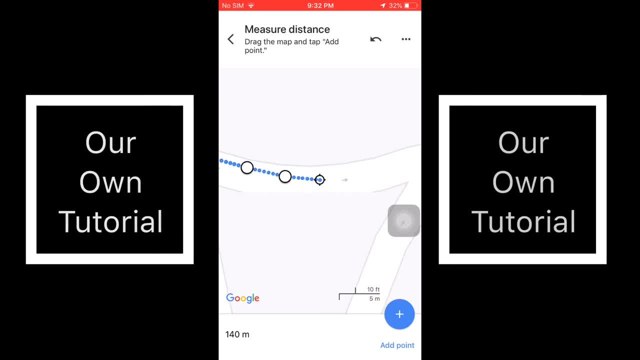 I am selecting this area or distance. you would notice that over here, below the Google, the distance is measuring. wait a minute. yeah, almost not. let me go a little bit further so that it will not touch to the other corner. here's perfect. no, okay, that's seems very easy. 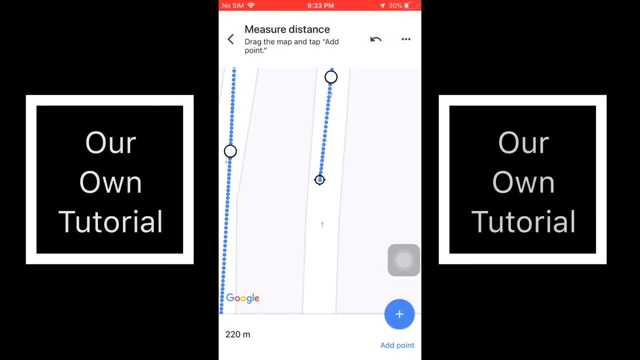 and let me go to fill the. and yeah, final, hear here. okay, so there is around 281. so, for example, you just made some mistakes and you want to remove this point over here. you can also remove it by just clicking this arrow. and yeah, it's almost on this side of your screen. nice, let's go ahead and do one more request: at z should be very easy to reach and the put a 지금 all over here. and yes, I found that on all the other encodings. so over here we'll press differently and click on over here if you have not been, for example, I already had it. finally, we will save by dragging the text to the board. you can also click on right upper left, on the right of the coder to go to print. Pour on and save the code that we just see what is the file download page. so the pic slash download in. 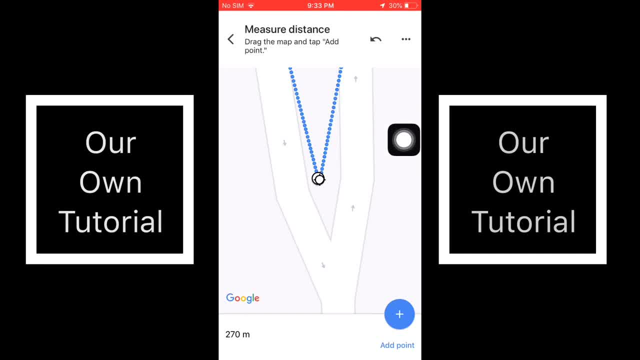 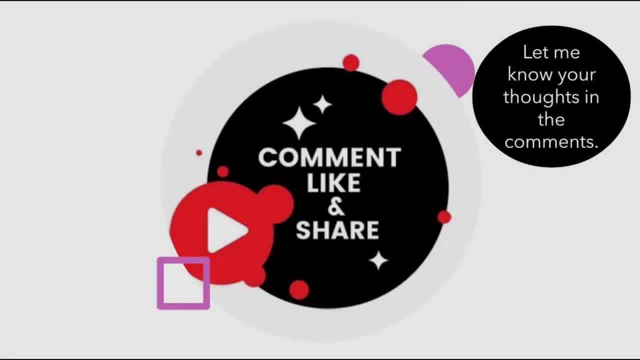 removed and you want to clear it, just click on here, then automatically everything will get clear and as it is same before, so very simple to do. well, that's it, finally. we just came to the end of video. and make sure, don't forget to comment and let me know your thoughts, whether this video work or not. bye, bye. have a good day, take care. 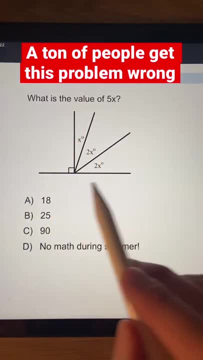 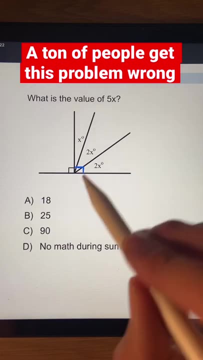 A ton of people get this problem wrong. It says: what is the value of 5x? and we have a diagram. we have a 90 degree angle right here, which means that this angle right here is also going to be 90 degrees, because this is a straight line. and since this angle right here is 90 degrees, that means 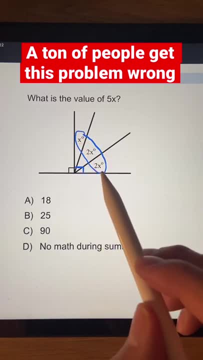 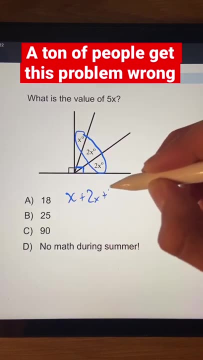 that if we were to add up all of these inside angles- x plus 2x plus 2x- all of them have to add up to 90 degrees. So let's go ahead and do that down here. So we have an x, we have a 2x and we 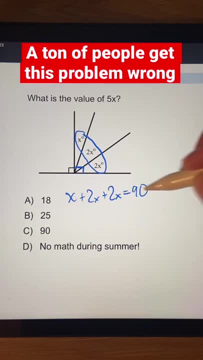 have a 2x and all of these angles added up has to equal 90 degrees. Okay, so now we can just add up like terms: x, 2x and 2x. that's going to be equal to 5x and we have it equals 90, and just like that. 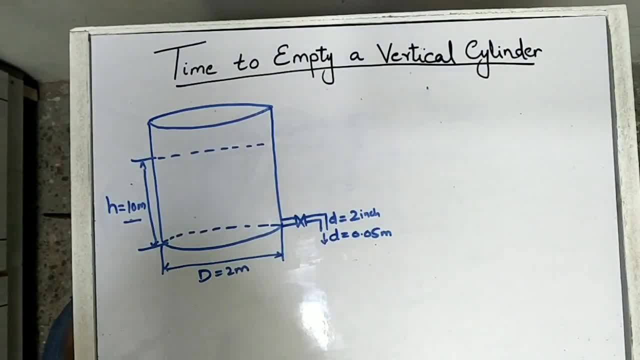 Welcome to the channel The Practical Study Guys. today we are going to calculate how much time will be required to empty a vessel through a drain point. For example, I have this vertical vessel. Its diameter is 2 meter and its height is 10 meter, and point to drain has a diameter of 2.